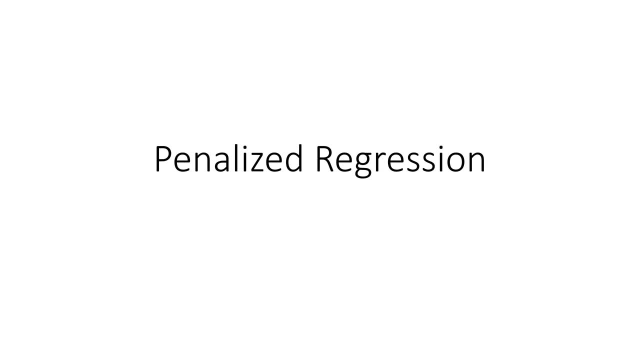 will be a very useful video for you. So first I am going to talk about the linear regression. So let us say we have this, a linear model which is y is equals to f of x plus epsilon. So we call this f of x as the mean function, which is equals to expected value of y, given x and this epsilon we 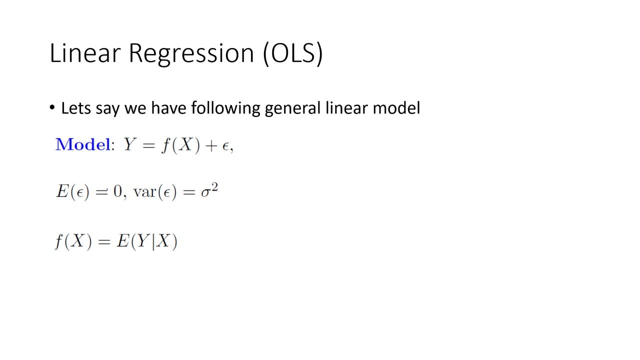 call as the random error. We know that expected value of epsilon is 0 and variance of epsilon is sigma squared. Now we are going to estimate this model using our data and we will get this y hat. y hat is equals to f of x hat, which is the estimated model of this. 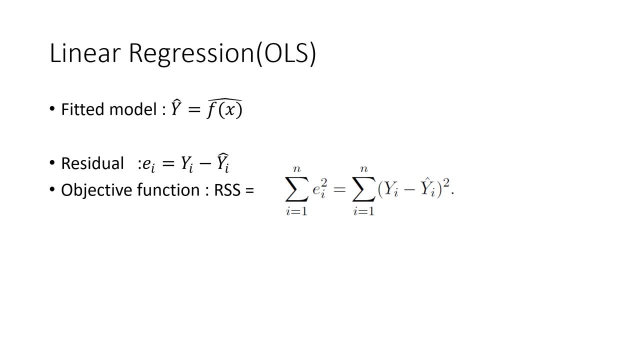 mean function. Usually this: the estimated value will not be equal to, it will not be equal to true value. In that case we will have a residual. Residual is equals to y high, y i minus y i hat. That means the difference between the observed value and the 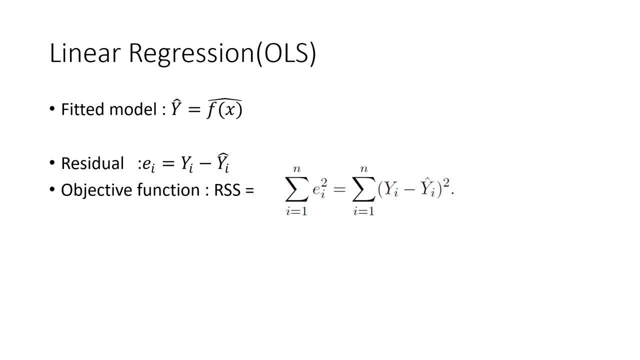 expected value. So our objective function is RSS, which is equals to residual sums of squares, which is equals to sum of ei squared, which is equals to a summation of y i minus y i hat squared. So our objective is to minimize this objective function or this cost function. 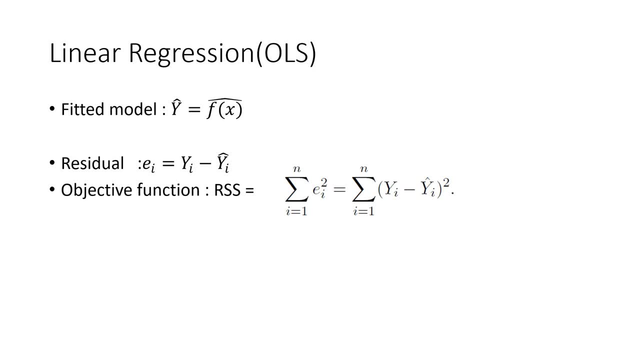 with respect to beta. So we will obtain our estimators of this true model. So by minimizing this objective function, we will obtain these OLS estimators, OLS regression model estimators. These estimators will be unbiased, but these estimators have high variance because of that. 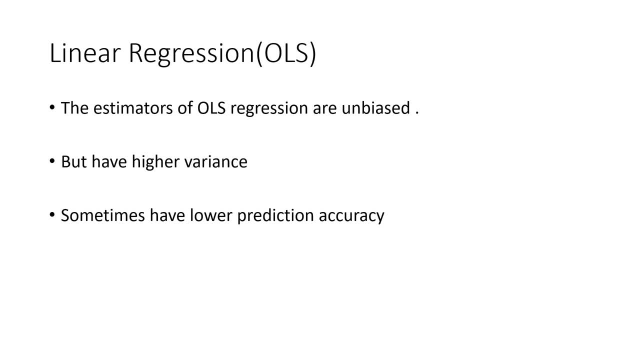 because of this high variability sometimes it will affect the prediction accuracy. That means because of this high variability sometimes the overall prediction accuracy of model will go down. So there is a problem. So if we have that kind of a situation then 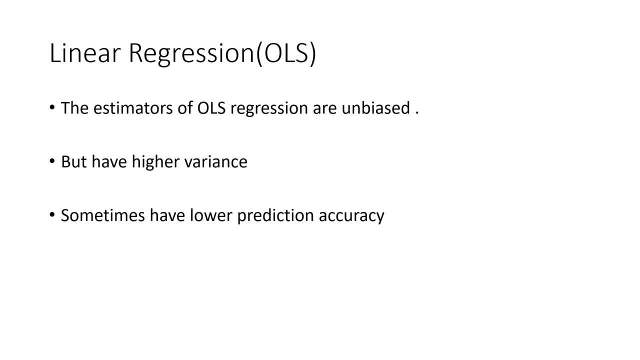 we can use this penalized regression. So in this penalized regression, what will happen is we are going to introduce some biased system system. So, by using this penalized regression, what will happen is we are going to introduce some biased system system. So in this penalized recreation. 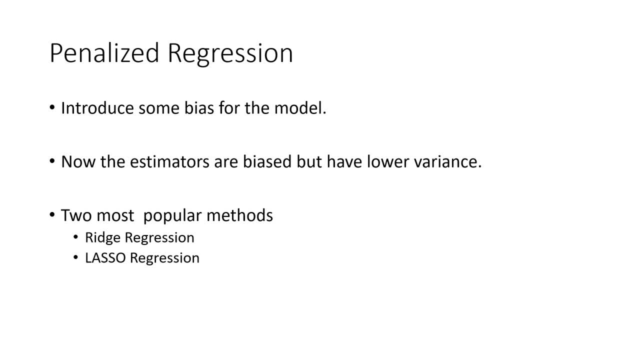 term to the model. So by introducing this bias term to the model, what will happen is these estimators are no longer unbiased. But the most important thing is that now these estimators have higher- sorry, lower- variance. So because of that, the prediction accuracy. 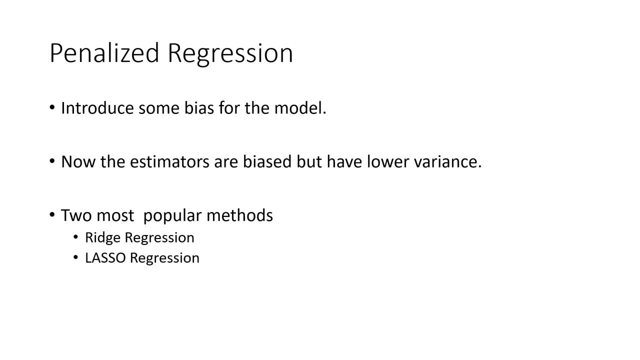 of this model will increase. So there are two most popular pin line regression techniques that people are using. The first one is a rich regression and the other one is a lasso regression. So the main difference in this rich regression and lasso- 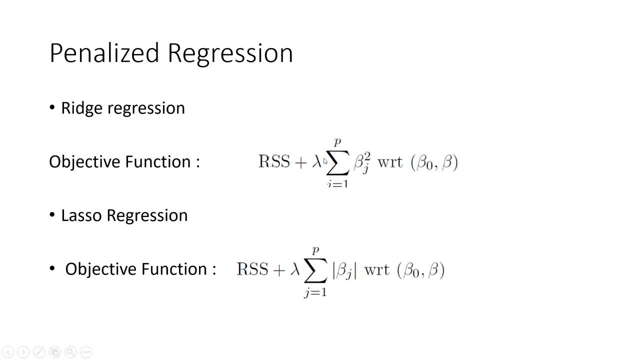 regression is due to the objective function. Now you can see, in this rich regression we have this RSS, which is equal to residual sums of squares, plus we have this penalty term times. This is L2 regularization term. this is L2 norm. So L2, we have this L2 norm. So now, 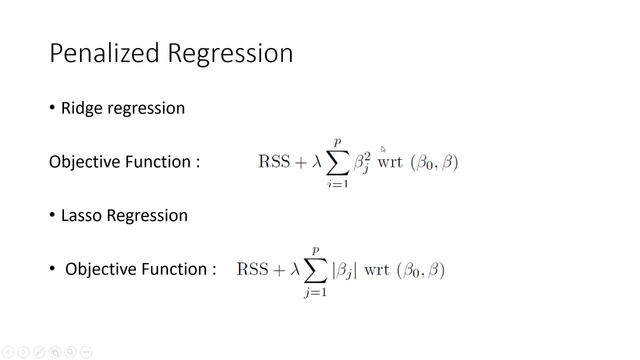 we are going to minimize the subjective function with respect to beta and in lasso regression. the difference is that instead of L2 norm we have this L1 norm here, which is equal to sum of these beta coefficients. So our goal is to minimize the subjective function. So 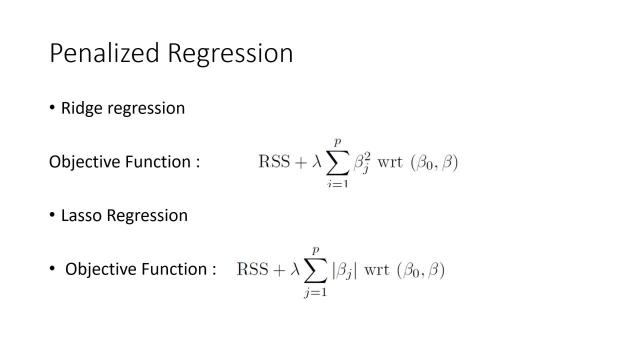 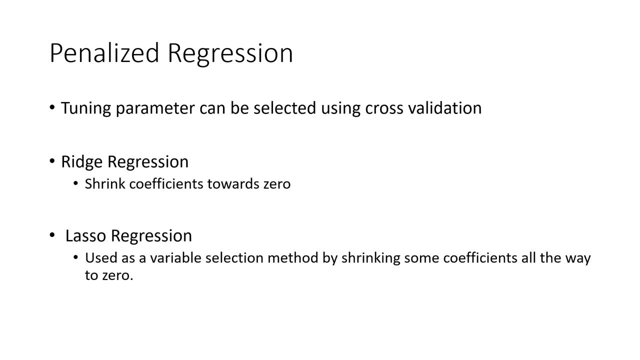 we have this function Once again. we have tau lambda. that is equal to tau lambda plus Po Safult. But to minimize the subjective function, if sqrt of0 is negative, then we can use what's called non undetermined derivative. Danny bound of2. so the respect to beta as 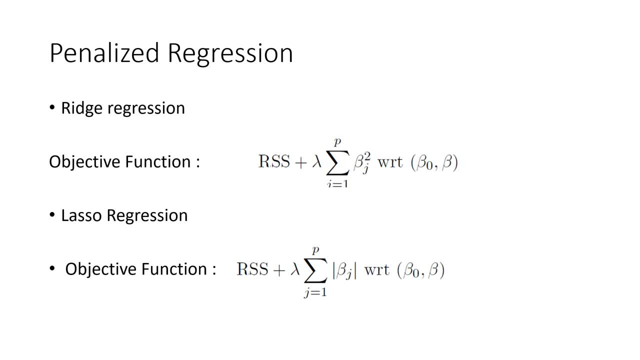 well as theta and theta also in one form. Again, we are going to minimize the subjective function, because negative value right now means that it's not positive and zamant who is not positive. So let us look at this Forever table. Then we look at the theta column and